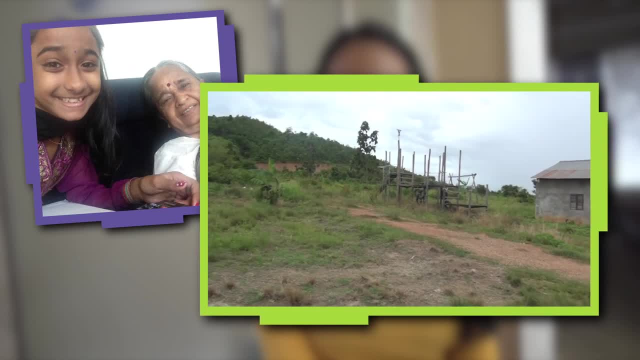 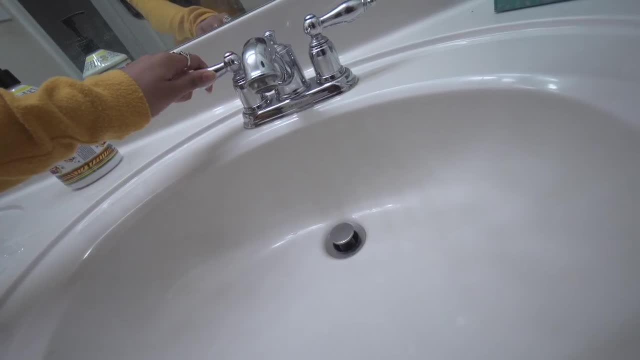 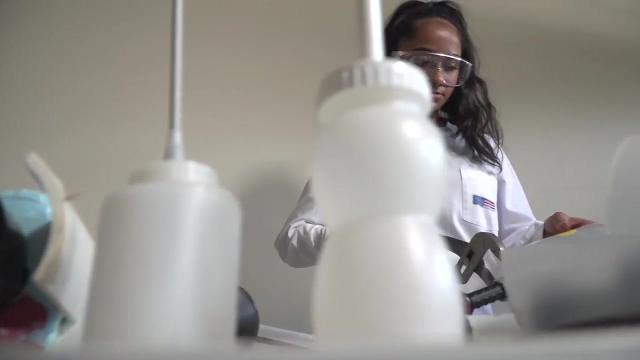 they experienced a water shortage. They only had enough water to drink and to cook. When this happened to my grandparents, I realized how close it hit to home. Unless we make minor changes in the way we use water, we may have to make huge compromises in the future. I wanted to find a way where I can save water at home. 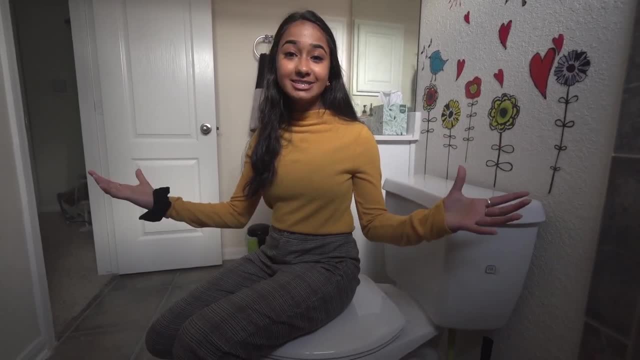 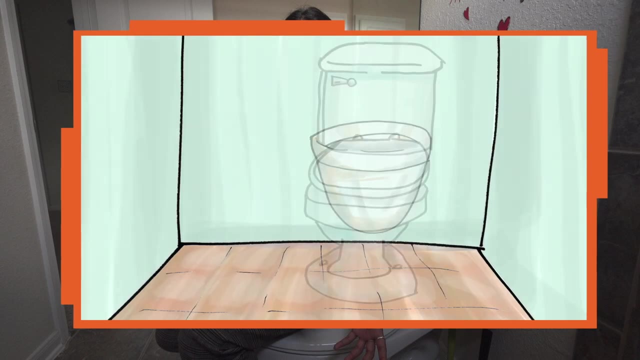 Nearly 30% of the water that you use in your entire house is used just in toilets. The toilet was invented in the late 1800s And we've been using the same design till today. There are two main parts to a toilet. 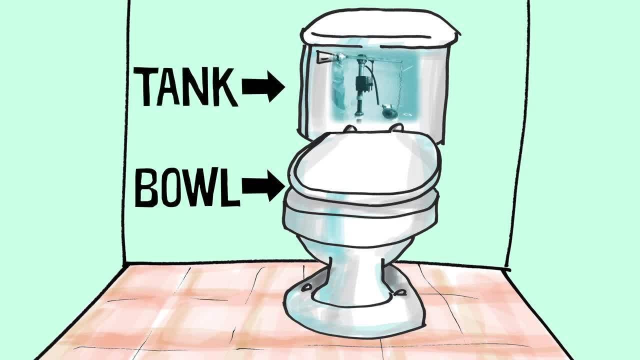 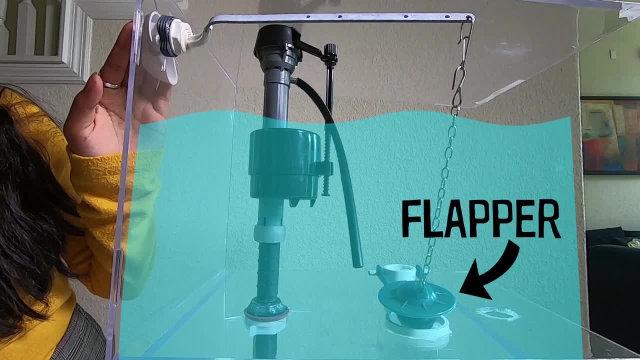 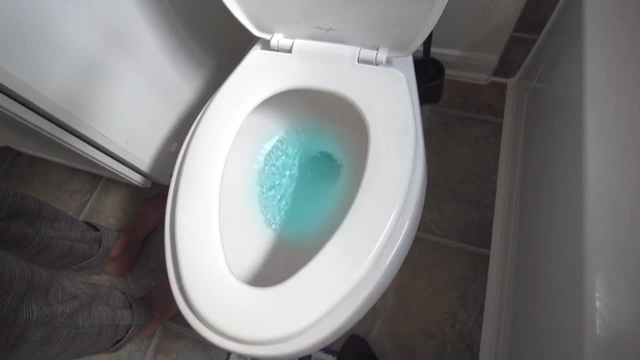 the bowl and the toilet tank. Let's look inside a typical toilet tank to see how it works. When you flush the toilet, this flapper gets pulled up, which will drain all the water in the tank and wash away the contents of the toilet bowl. And once you close the flapper, 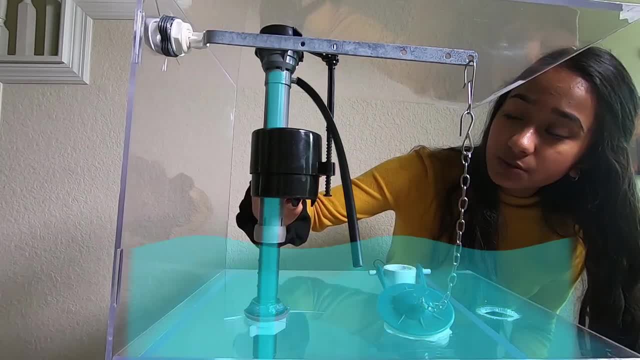 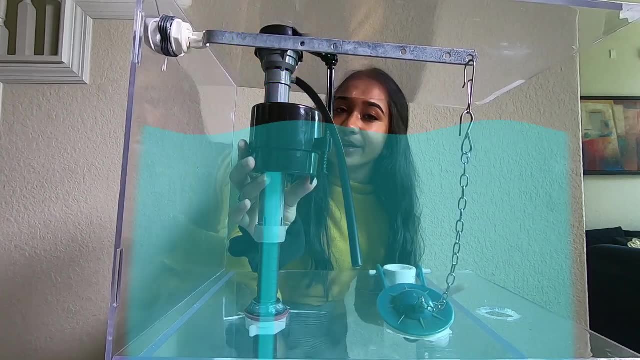 the water will flow from this tube. This float will be the water that will be used to clean the toilet bowl. And once you close the flapper, the water will flow from this tube. This float will be the water that will come up. The valve will close, which will stop the fresh water from flowing into. 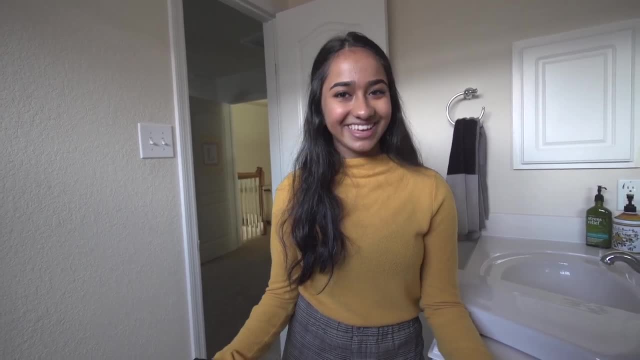 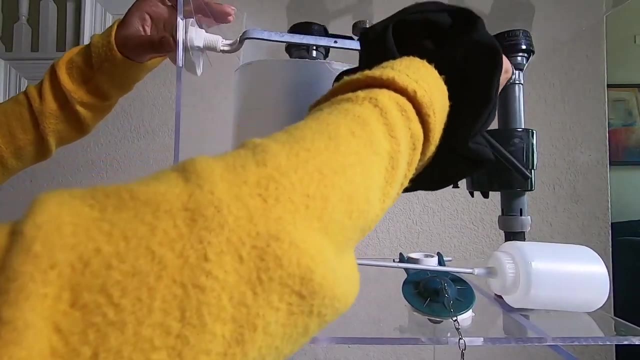 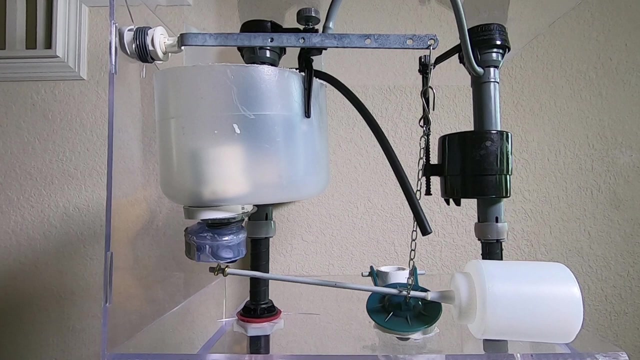 the tank And then the toilet is ready to be flushed again. The toilet has been around for over 100 years And my invention improved the previous invention. This is my invention, Aria. The main part of Aria is a mini tank inside the main tank. 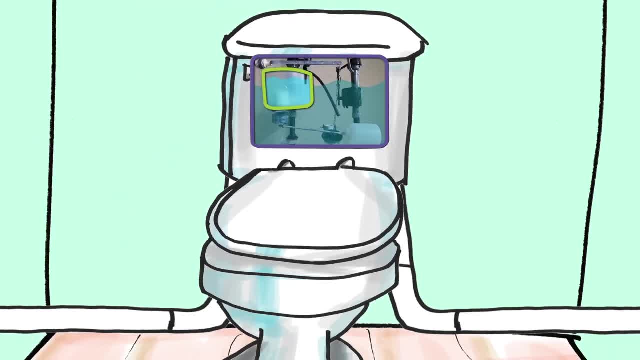 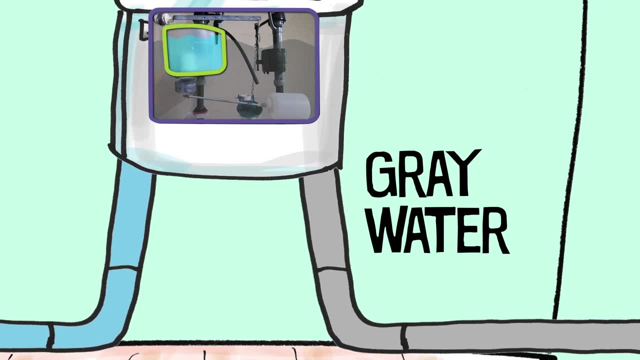 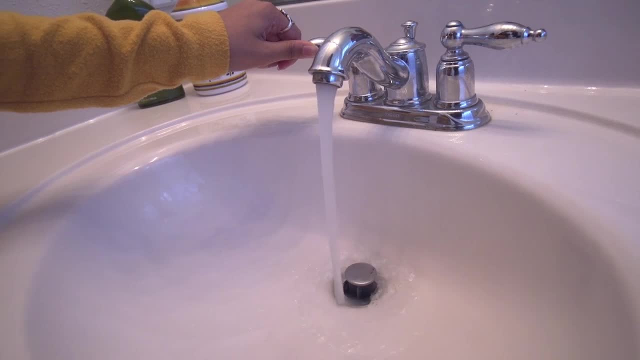 of a toilet. This improvement allows a regular toilet to use two sources of water: fresh water and, most importantly, grey water, which is recycled water. Grey water is the water that goes down the drain After you wash your hands, after you wash the dishes, after you wash your clothes, after you take a shower. that's all grey water. 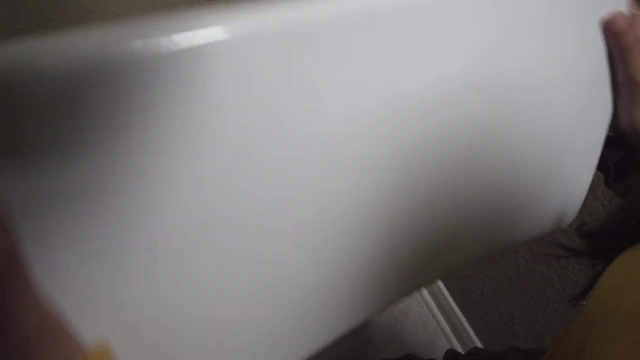 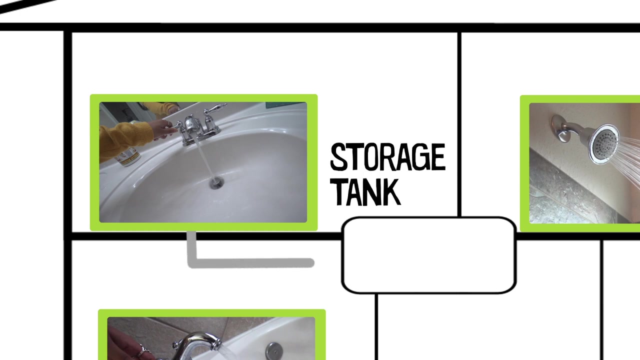 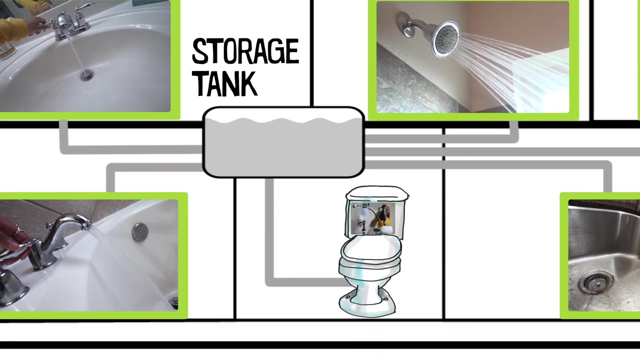 Grey water is not the fresh water that you drink. The water that we use in toilets doesn't have to be fresh water. With my invention, you need a storage tank to collect grey water from around the house. If a toilet has my invention installed, it would use grey water from the storage tank.